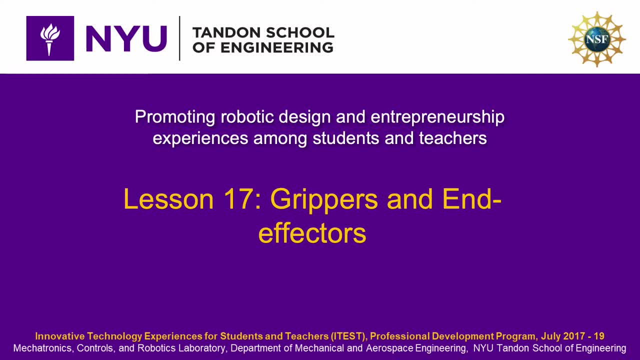 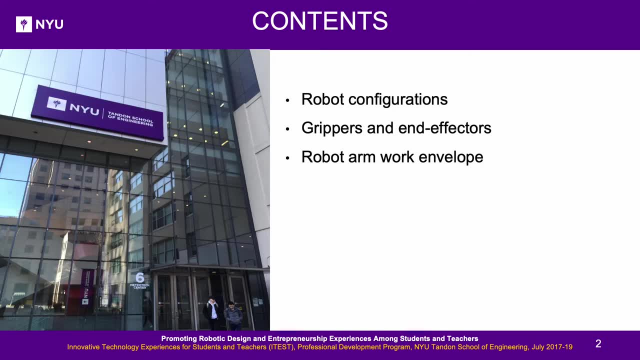 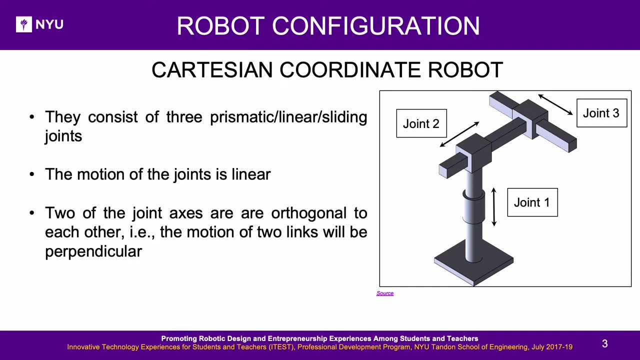 Lesson 17.. Grippers and End Effectors. Contents. The topics covered in this lesson are Robot Configurations, Grippers and End Effectors, Robot Arm Work Envelope. Robot Configuration- Cartesian Coordinate Robot. They consist of three prismatic, also called as linear or sliding joints. The motion of the joints is linear. 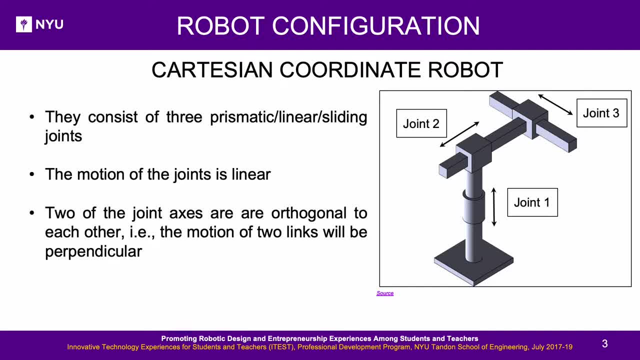 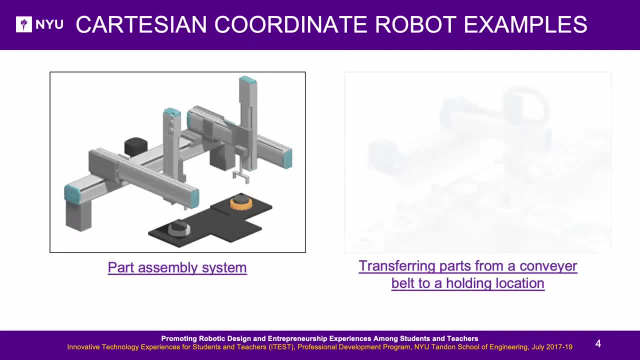 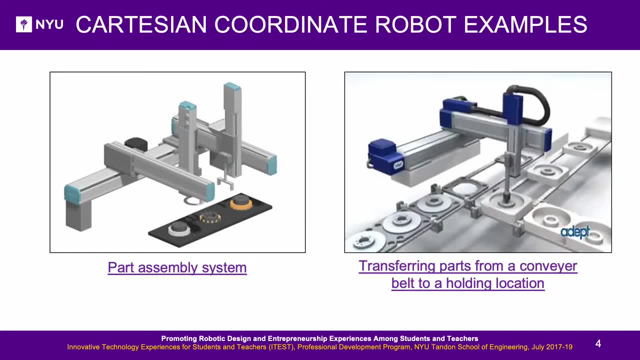 In this configuration at least two of the joint axes are orthogonal to each other, That is, the motion of two links will be perpendicular to each other. Here we can see the examples of Cartesian Coordinate Robots. In the first example there is a part assembly system. The second example shows a conveyor belt. 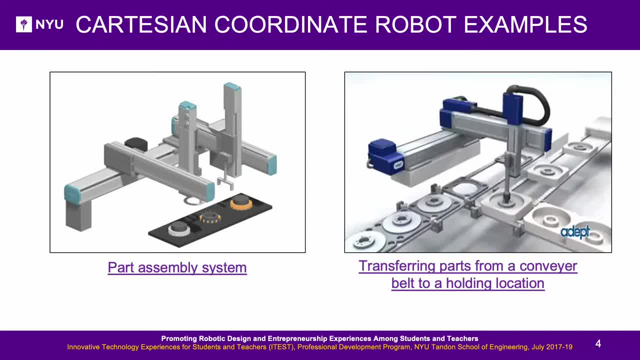 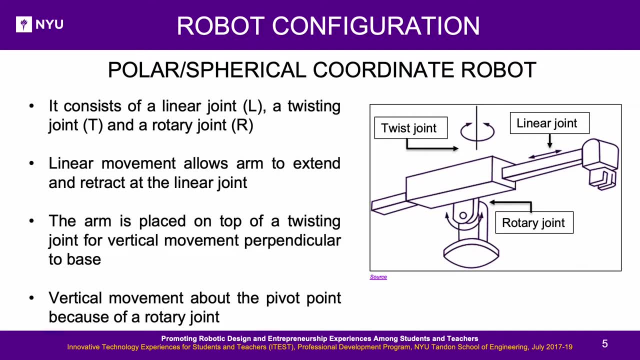 with parts being transferred by a Cartesian system, Polar or Spherical Coordinate Robots. It consists of a linear joint L, a twisting joint T and a rotary joint R. The linear movement allows arm to extend and retract at the linear joint. 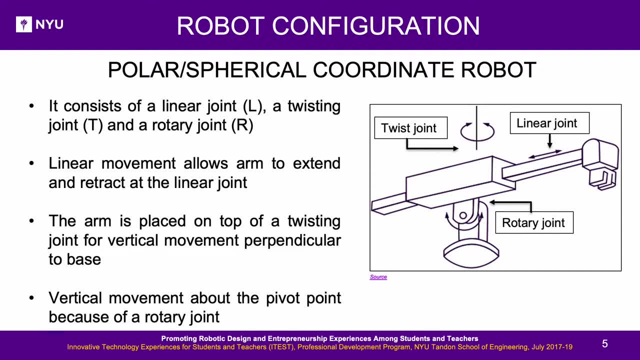 The arm is placed on top of a twisting joint for vertical movement perpendicular to base of the robot. There is a vertical movement about the pivot point because of the presence of a rotary joint. Here we can see the examples of Polar Coordinate Robots. 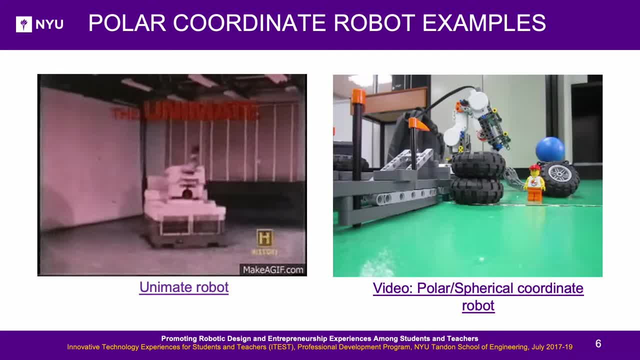 In the first example there is a part assembly system. The second example shows a polar coordinate system. In the first example we can see the Unimate Robot. The second example shows a conveyor belt, a robot project with a polar coordinate system. 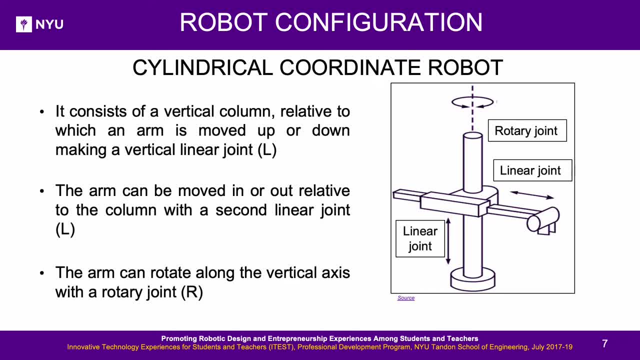 It consists of a vertical column relative to which an arm is moved up or down, making it a vertical linear joint L. The arm can be moved in or out relative to the column. with a second linear joint L. The arm can rotate along the vertical axis with a rotary joint R. 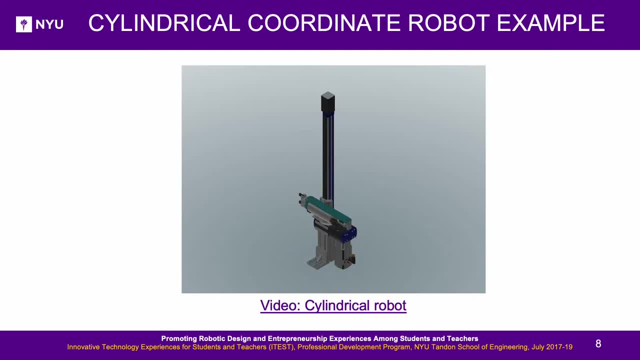 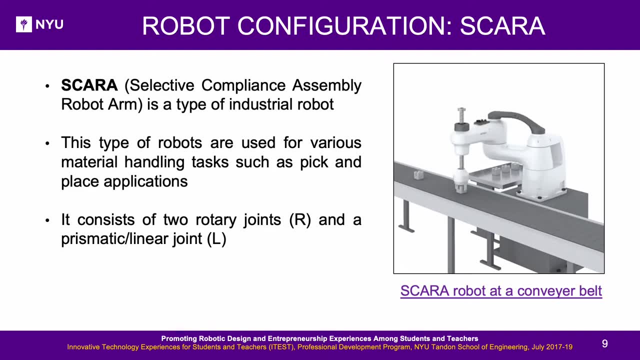 Here we can see an example of Cylindrical Coordinate Robot Robot Configuration S-C-A-R-A SCARA Selective Compliance Assembly Robot Arm is a very common type of an industrial robot. This type of robots are used for various material handling tasks, such as pick and place. 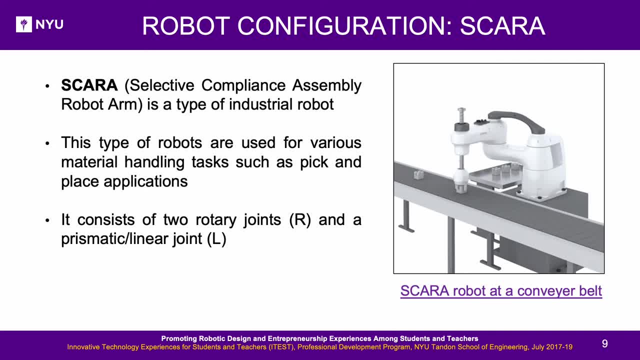 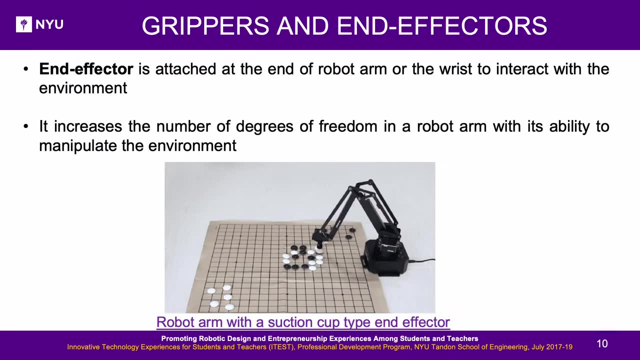 applications. It consists of two rotary joints R and a linear joint L. Here in the example we can see the SCARA robot performing a pick and place operation on a conveyor belt, Grippers and End Effectors. End Effector is attached at the end of robot arm or the wrist to interact with the environment. 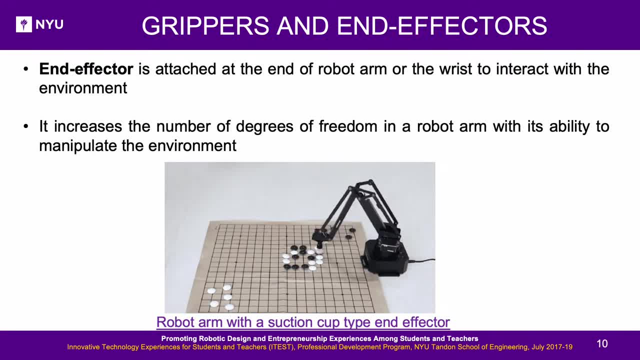 It increases the number of degrees of freedom in a robot arm, as it increases the ability of the robot to manipulate the environment in additional ways. Here we can see a manipulator with an gripper attached to it playing the Chinese chess with a human. 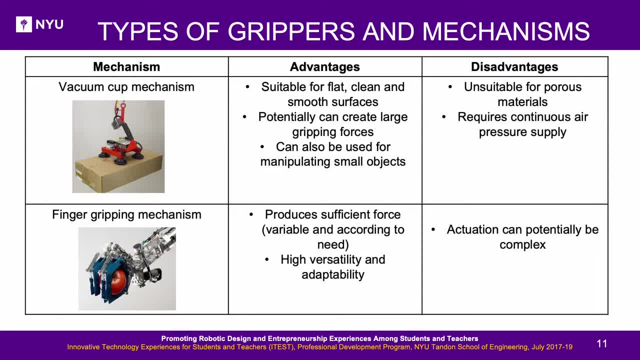 Types of Grippers and Mechanisms. There are various types of gripping mechanisms. They are: Vacuum Cup Mechanism. Motor Gripping Mechanism. Pneumatic Powered Grippers. Hydraulic Powered Grippers. Motor Actuation- Parallel or Translational Mechanism. Angular or contour mechanism. The 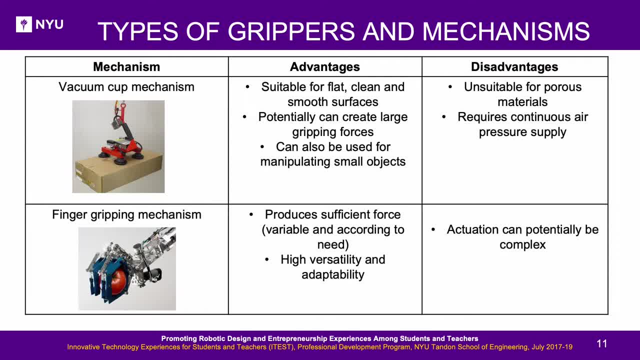 advantages and disadvantages of using the Vacuum Cup Mechanism are: Advantages: suitable for flat, clean and smooth surfaces. Potentially can create large gripping forces. Can also be used for manipulating small objects. Disadvantages: Unsuitable for Porous Materials To shelf the gear of the machine. Disadvantages to smoothing by using vacuum for motionAAA or impossible for smooth surface to handle small objects. Disadvantages to maneuver small objects through lap. Easy to manage the impact force without an across. 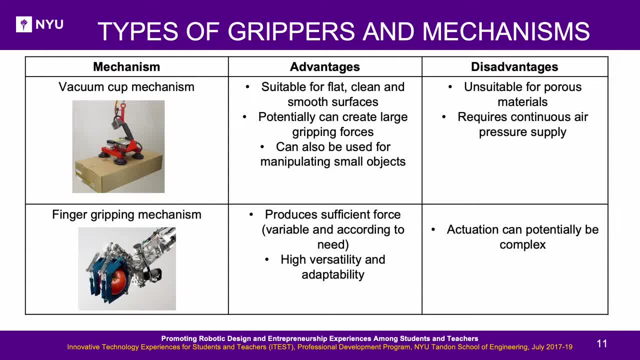 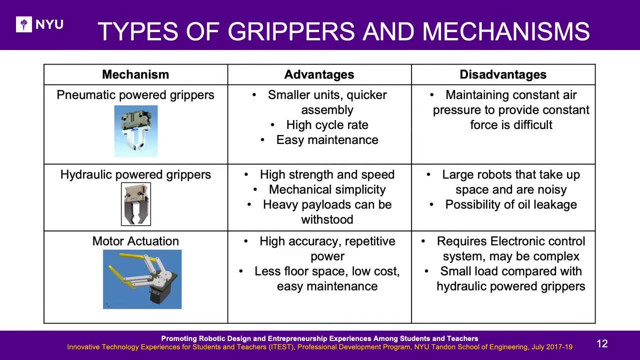 materials: Requires continuous air pressure supply. The advantages and disadvantages of using the finger gripping mechanism are: Advantages: Produces sufficient force, variable and according to need. High versatility and adaptability. Disadvantages: Actuation can potentially be complex. The advantages and disadvantages of using the pneumatic powered: 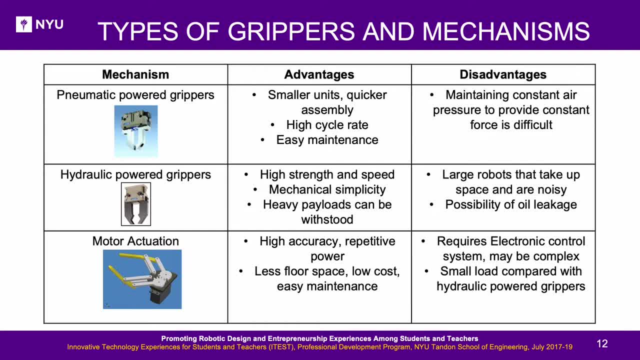 grippers are Advantages: Smaller units, quicker assembly, High cycle rate, Easy maintenance. Disadvantages: Maintaining constant air pressure to provide constant force is difficult. The advantages and disadvantages of using the hydraulic powered grippers are Advantages: High strength and speed. Mechanical simplicity. Heavy payloads can be withstood. 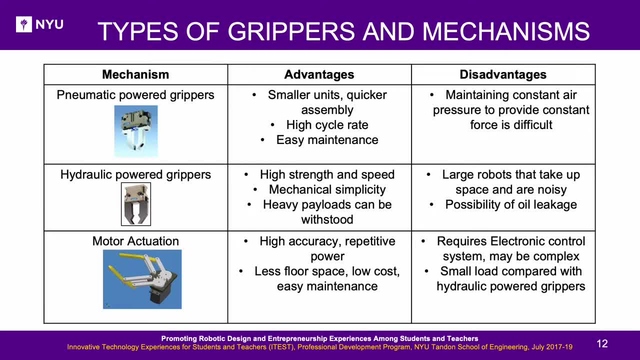 Disadvantages: Large robots that take up space and are noisy, Possibility of oil leakage. The advantages and disadvantages of using the motor actuation are Advantages: High accuracy, Repetitive power, Less floor space, Low cost, Easy maintenance. 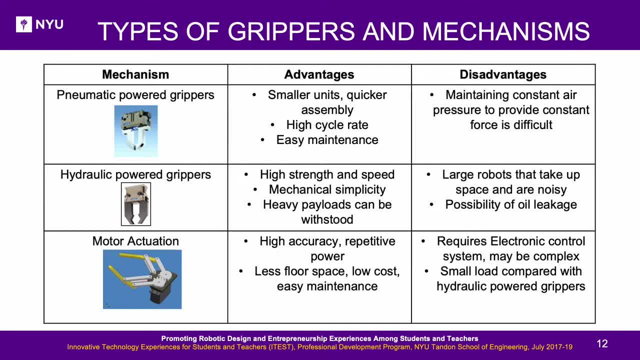 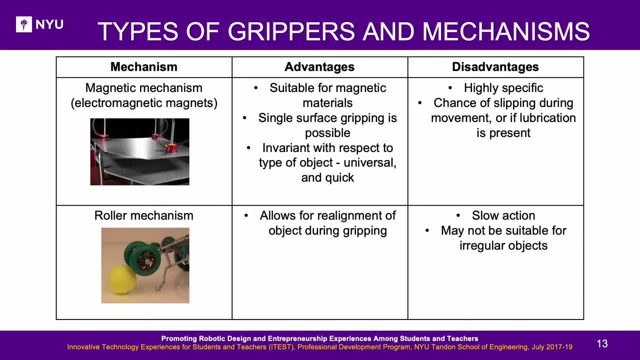 Disadvantages: Requires: electronic control system May be complex. Small load compared with hydraulic powered grippers. The advantages and disadvantages of using the magnetic mechanism are: Advantages Suitable for magnetism, Magnetic materials. Single surface gripping is possible, Invariant with respect to type of object. 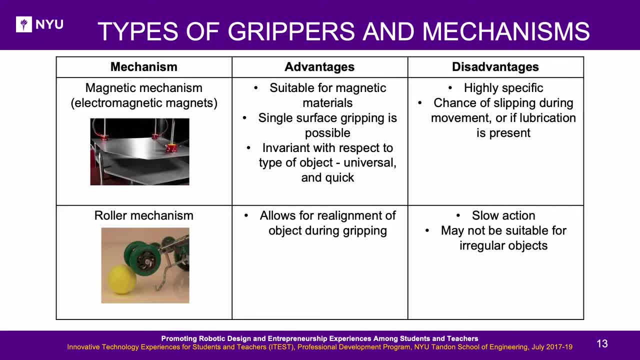 Universal and quick Disadvantages. Highly specific Chance of slipping during movement or if lubrication is present. The advantages and disadvantages of using the roller mechanism are: Advantages: Allows for realignment of object during gripping. Disadvantages: Slow action. 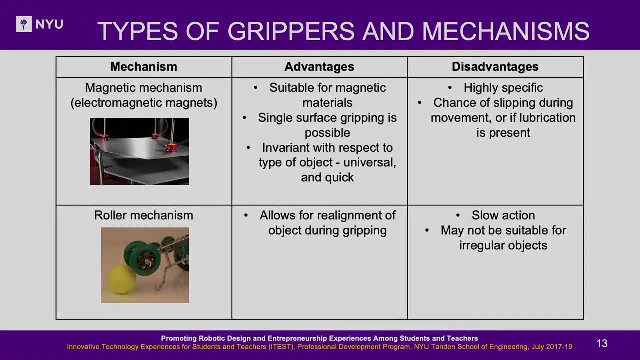 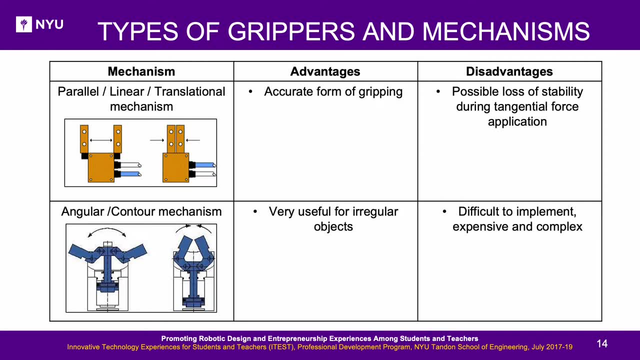 May not be suitable for irregular objects. The advantages and disadvantages of using the parallel or linear or translational mechanism are: Advantages: Accurate form of gripping. Disadvantages: Possible loss of stability during tangential force application. The advantages and disadvantages of using the angular or contour mechanism are: 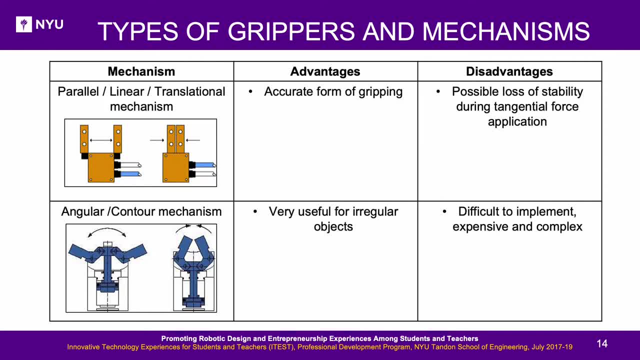 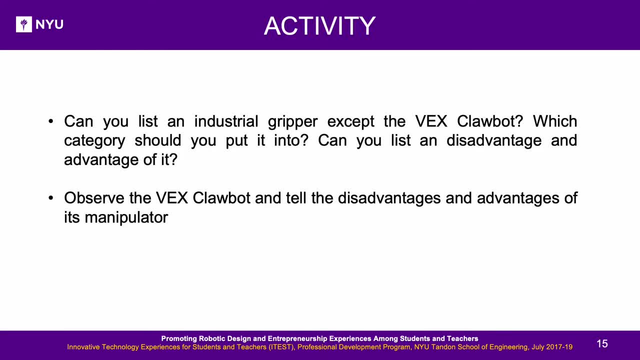 Advantages: Very useful for irregular objects. Disadvantages: Difficult to implement, Expensive and complex Activity. Can you list an industrial gripper except the Vex Clawbot? Which category should you put it into? Can you list an disadvantage and advantage of it? 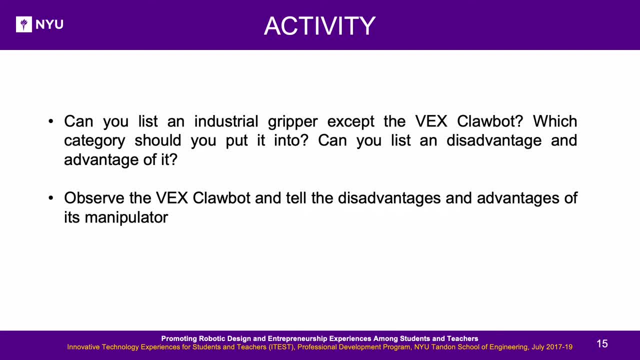 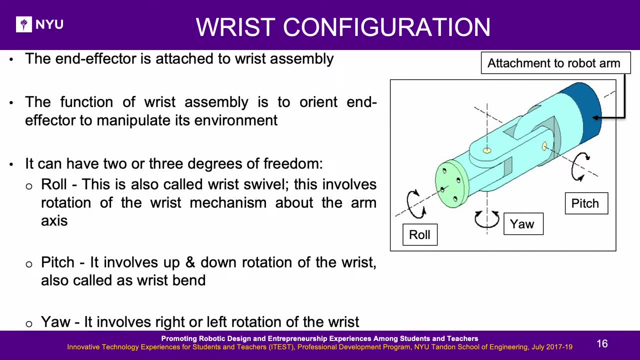 Observe the Vex Clawbot and tell the disadvantages and advantages of its manipulator Wrist configuration. The end effector is attached to wrist assembly. The function of wrist assembly is to orient end effector to manipulate its environment. It can have 2 or 3 degrees of freedom. 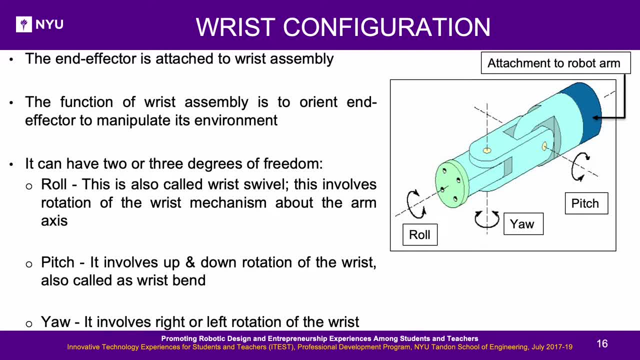 Role. This is also called wrist swivel. This involves rotation of the wrist mechanism about the arm axis Pitch. It involves up and down rotation of the wrist, Also called as wrist bend Yaw. It involves right or left rotation of the wrist. 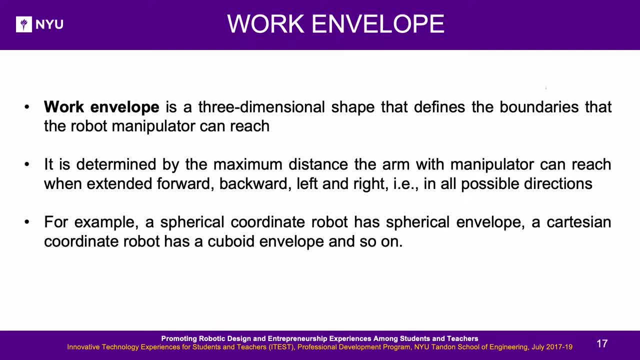 Work envelope. Work envelope is a three-dimensional shape that defines the boundaries that the robot manipulator can reach. It is determined by the maximum distance the arm with manipulator can reach when extended forward, backward, left and right, That is, in all possible directions. 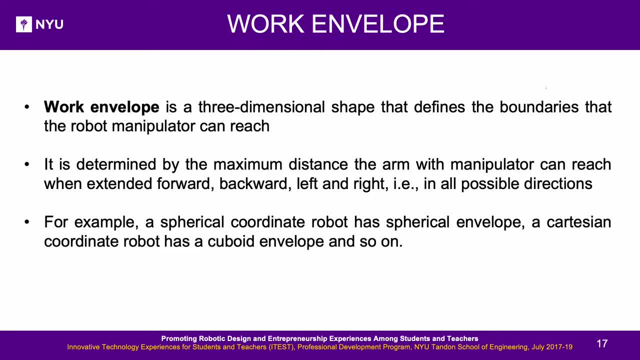 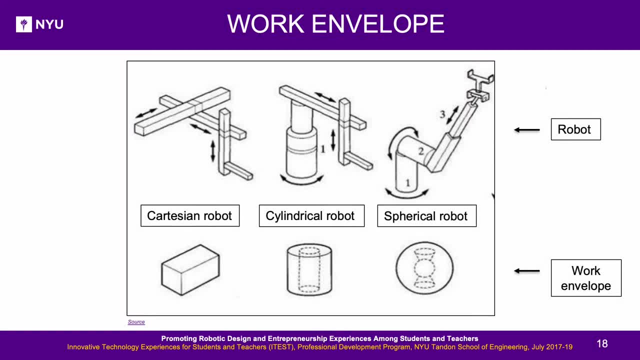 For example, a spherical coordinate robot has spherical envelope, A Cartesian coordinate robot has a cuboid envelope, and so on. The work envelope for Cartesian, cylindrical and spherical robots are shown in the following figure: Cartesian robot has a rectangular work envelope. Cylindrical robot has a rectangular work envelope. 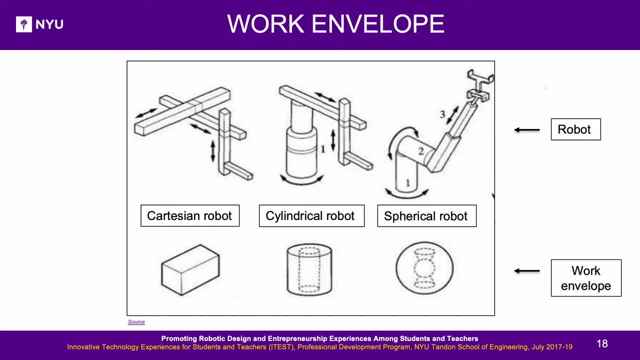 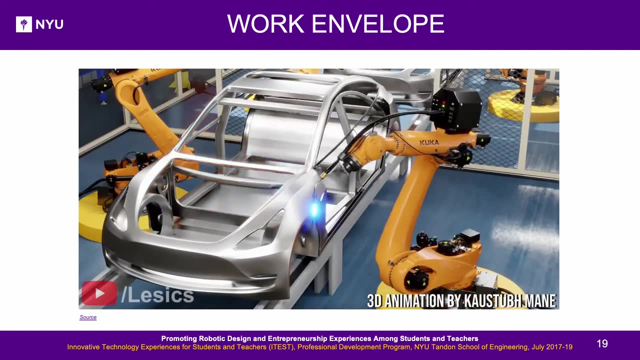 Spherical robot has a rectangular work envelope. The dotted area within the envelope is the area where the robot end effector cannot reach, and so is the area outside the solid line. Robots are designed based on the work envelope required. The volume the end effector of this robot is able to reach is known as the work envelope. 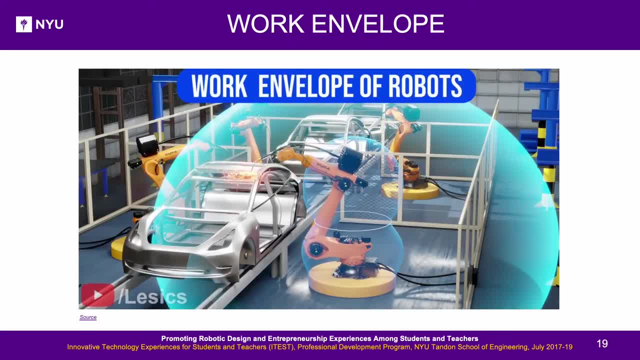 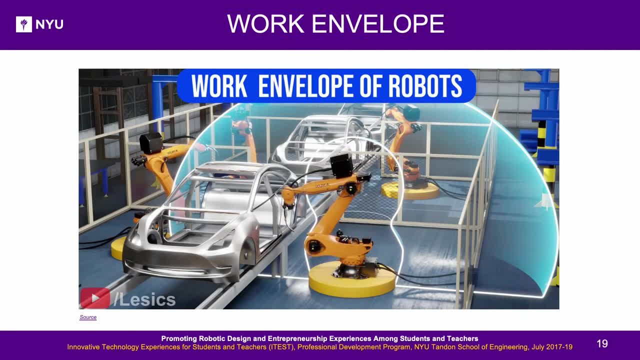 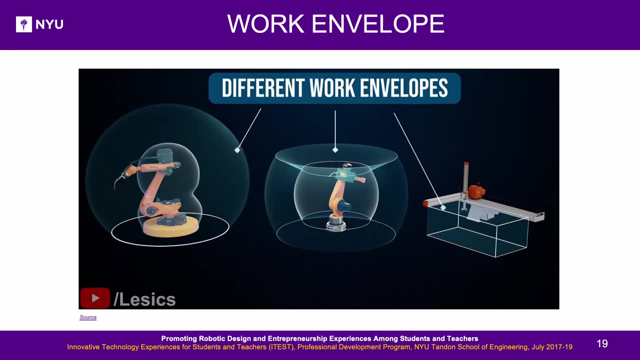 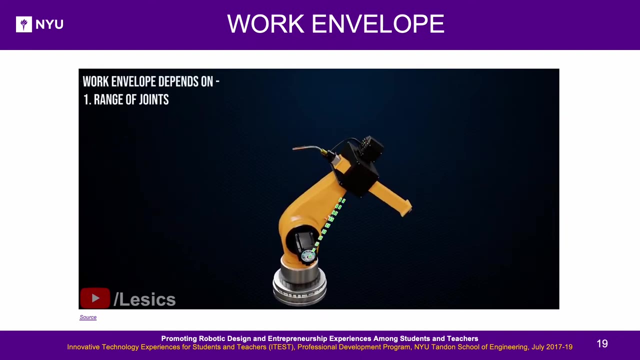 For example, for this robot shown the blue shade volume is the work envelope. Let's learn more about this crucial concept of robotics. The work envelope is different for different robots. A robot's work envelope depends on three physical characteristics. The first one is the range of the robot's joints. 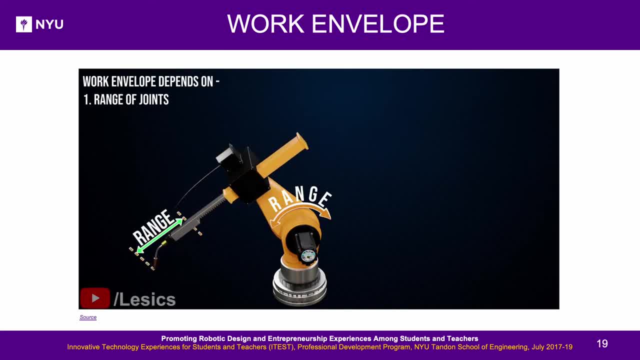 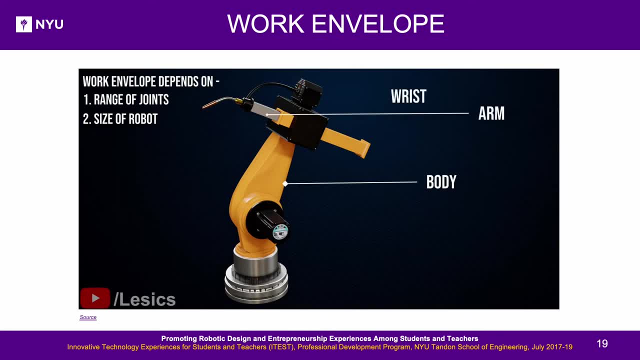 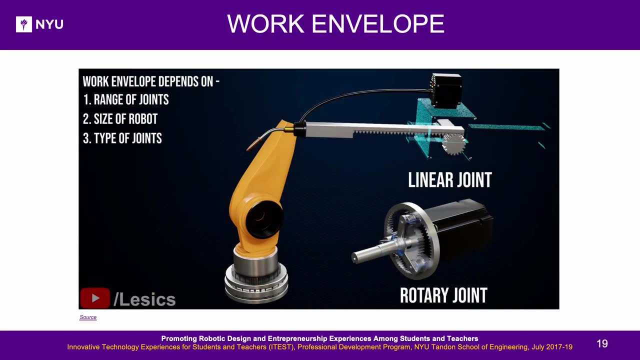 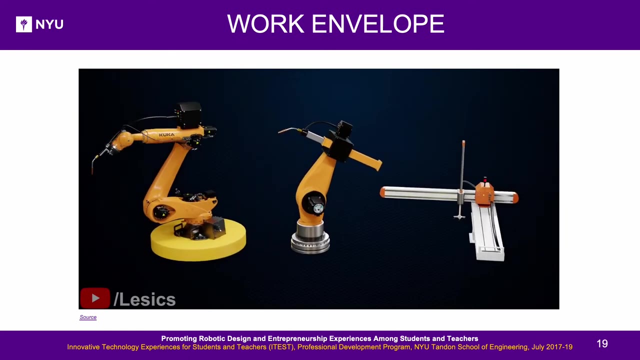 Both the linear and angular range of a robot is illustrated here. The second characteristic is the size of its body. The third characteristic is the size of the robot's arm and wrist. The last characteristic is the type of joints. Different work envelopes are created by modifying these three characteristics. 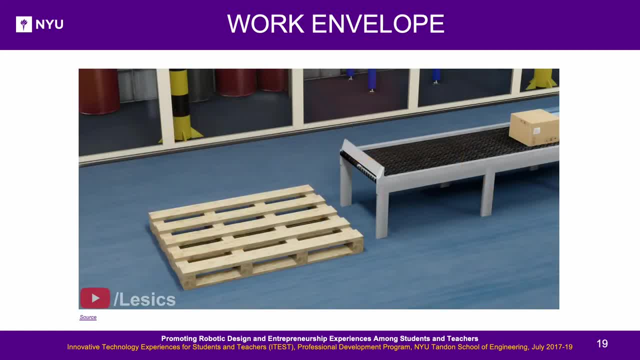 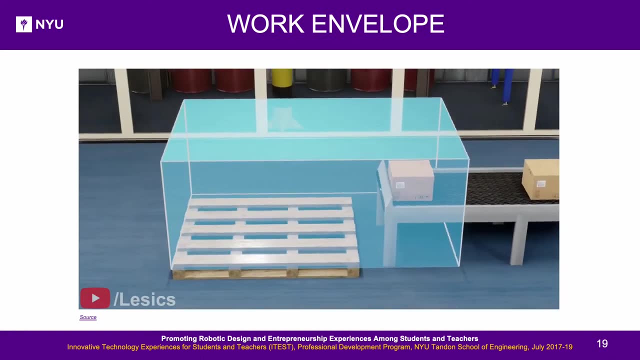 Let's understand these concepts with the help of a robot design challenge. Suppose we have to collect some boxes from a conveyor belt and place them in this highlighted location. The work envelope required for the robot is obviously rectangular in shape. Can you guess what type of robot configuration is the best fit to complete this task? 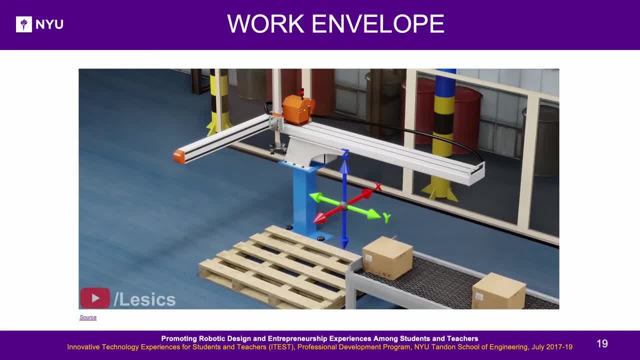 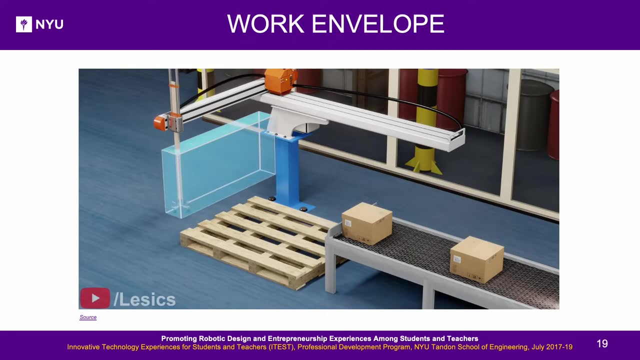 Yes, you'd need a robot with linear motions in all three directions inside this volume. This robot has three linear joints to accomplish movement in the X, Y and Z directions. This robot's end effector can pick up the object anywhere inside this rectangular work envelope. 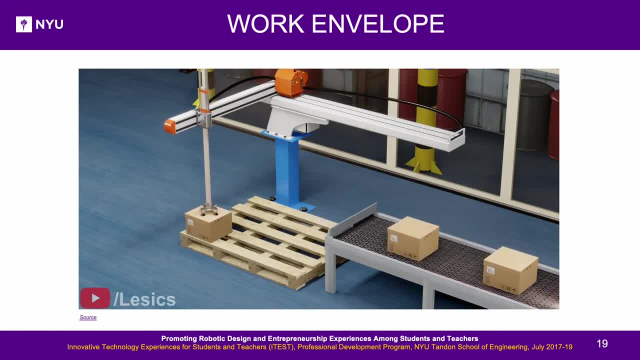 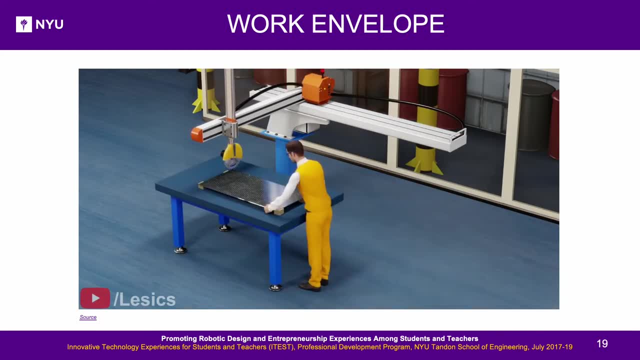 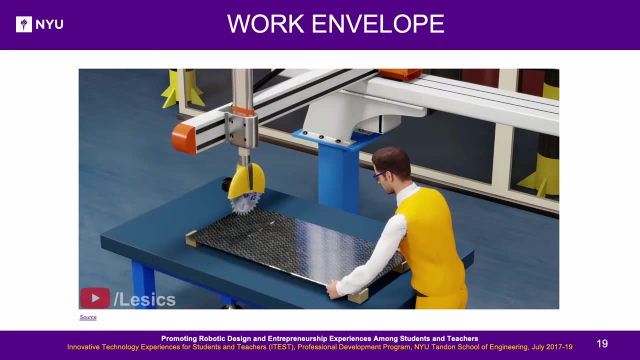 move in all three axes and place it as needed. These kinds of robots are called Cartesian robots. Now let's consider the same robot, but this time it's using a different end effector, a metal cutter. Here, due to the nature of the work, the operator has to be inside the work envelope we designed. 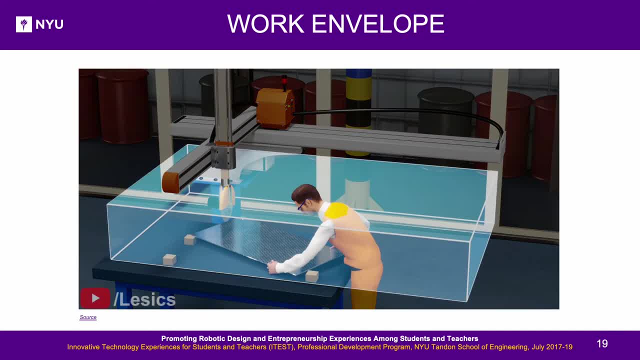 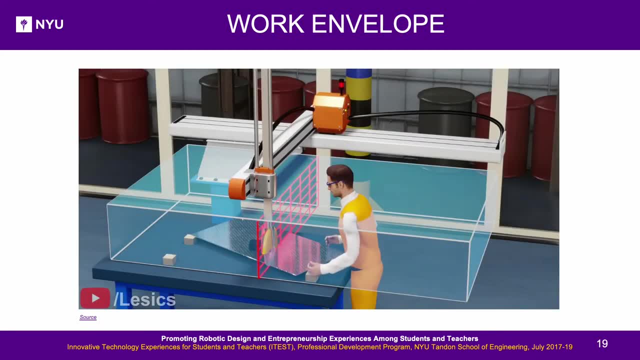 This can be defined earlier- which can be highly dangerous For safety purposes. you won't want this new end effector to go near the operator's hand. In short, you have to block the robot's movement in the Y direction after this red plane. 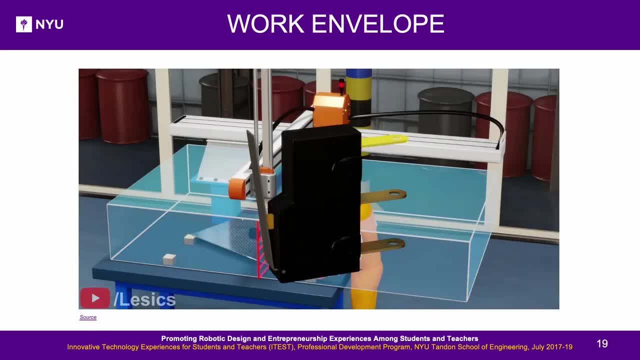 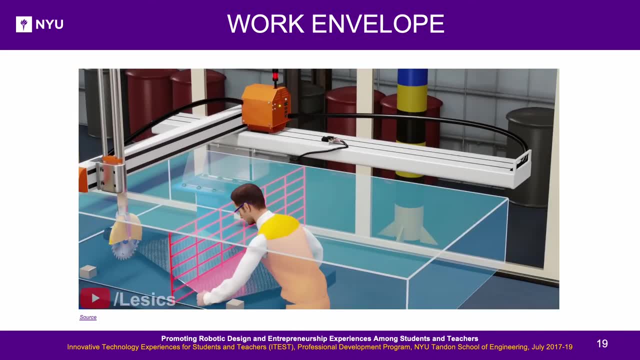 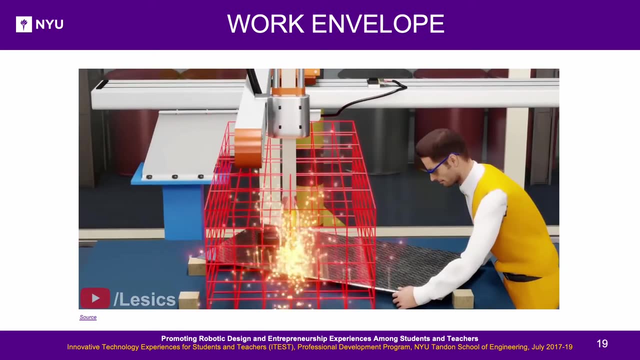 To achieve this end, engineers often restrict the movement of the robot by using electromechanical limit switches, which creates a border beyond which the robot cannot go in any given conditions. In short, even though the work envelope is huge, this robot will be able to work only within this red volume. 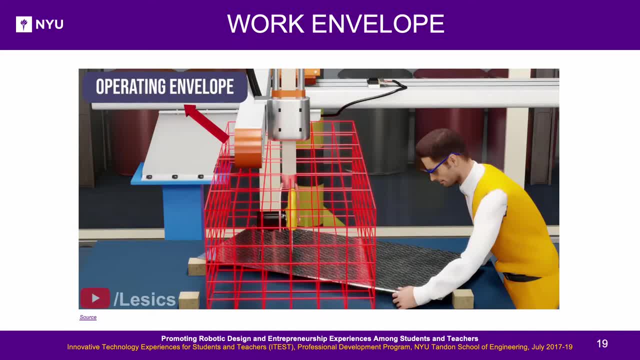 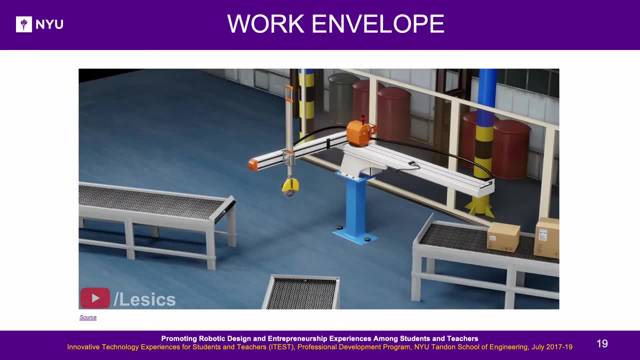 This new red volume is called an operating envelope. Let's move to our next robot and study a different work envelope. Let's assume that the robot has to move these boxes from one conveyor belt to another. The work envelope needed for this task is obviously cylindrical in nature. 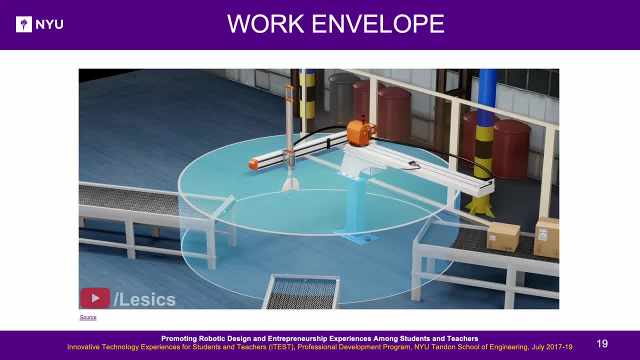 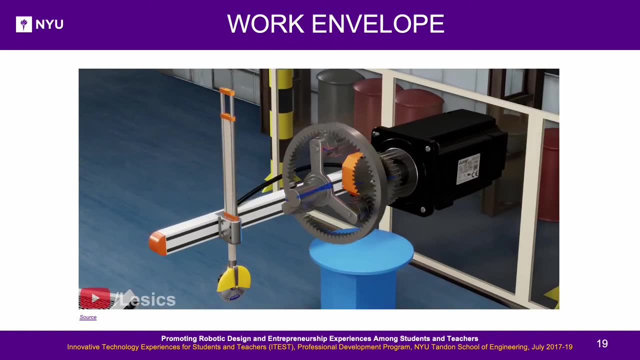 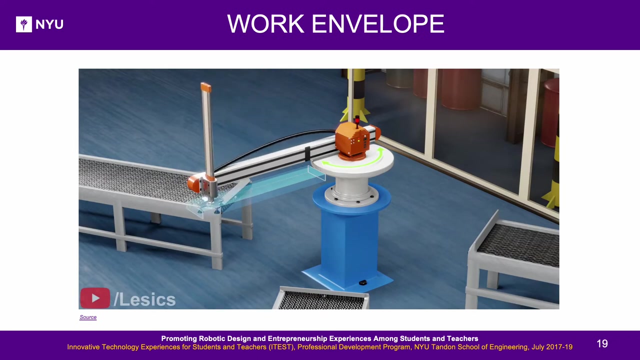 Can you suggest some design modifications to the previous robot to achieve the new work envelope? To attain the cylindrical volume we need two linear movements and one rotary movement. Simply replace one linear joint from the Cartesian robot with a rotary joint. Now the robot can rotate 360 degrees on its central axis. 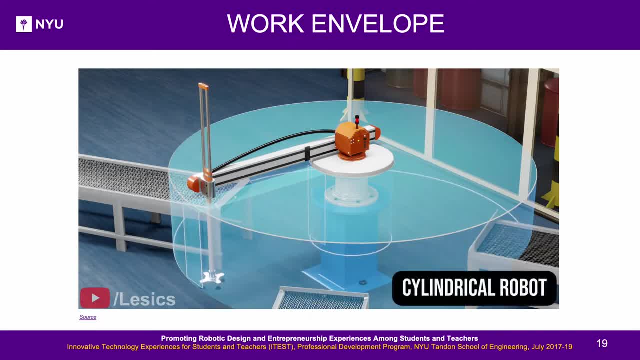 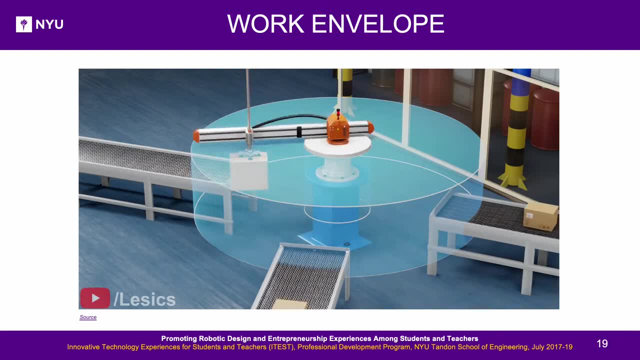 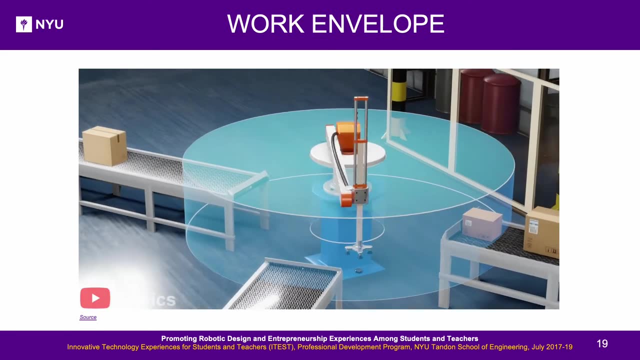 These kinds of cylindrical robots are mainly used to work as mediators between two or three massive machines to transfer an object from one station to another. If you observe carefully, you can see that the work envelope here is not a solid cylinder. It has a dead zone at the center. 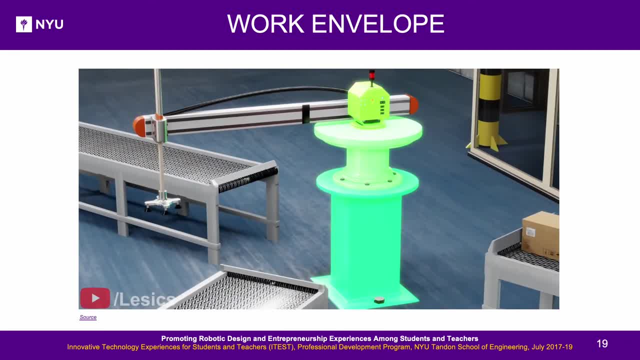 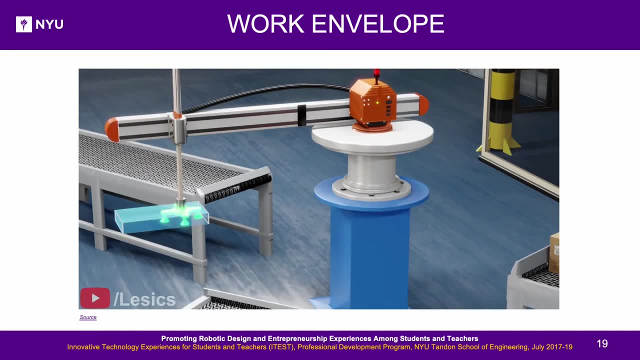 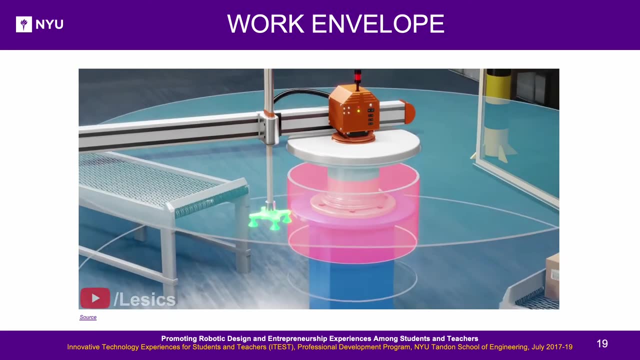 Can you tell why This dead zone is due to the robot body's physical limitation? In this case, you can see that the robot's arm can retract only up to its body and not beyond that. Thus, a dead zone volume will always be inside the cylindrical robot's work envelope. 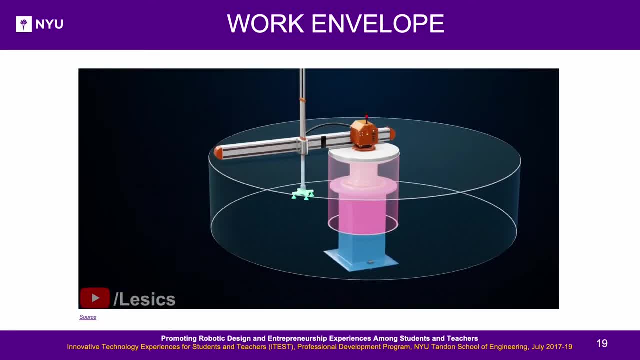 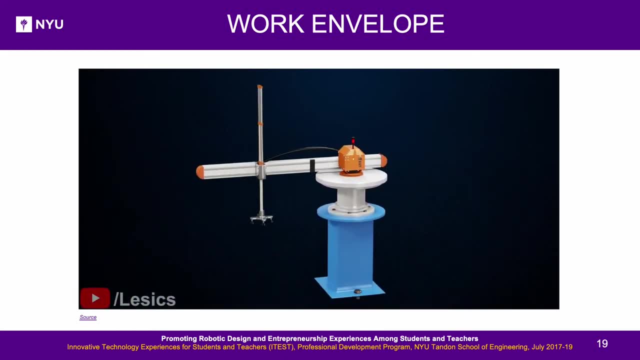 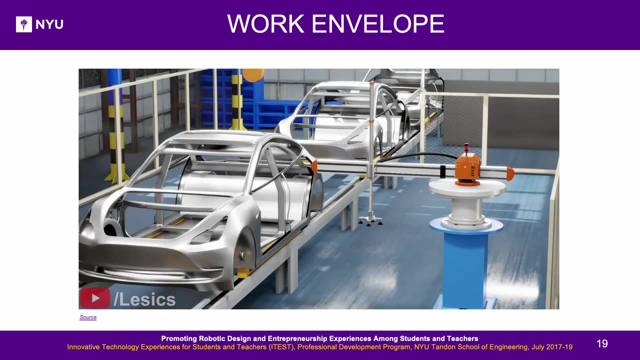 However, such dead zones are not present inside the Cartesian robot's work envelope. With a simple design modification, we can convert this cylindrical robot into a more versatile robot which does tasks like welding this car chassis together. For this task, the robot has to turn at different complicated angles. 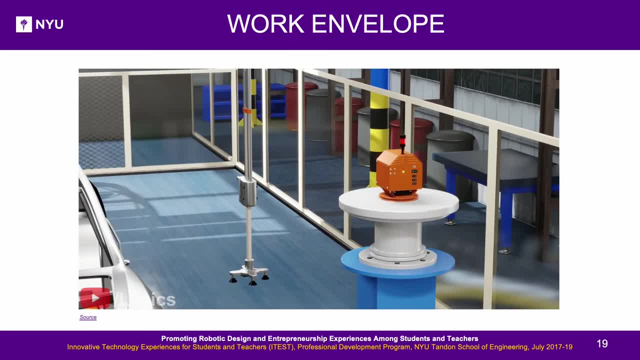 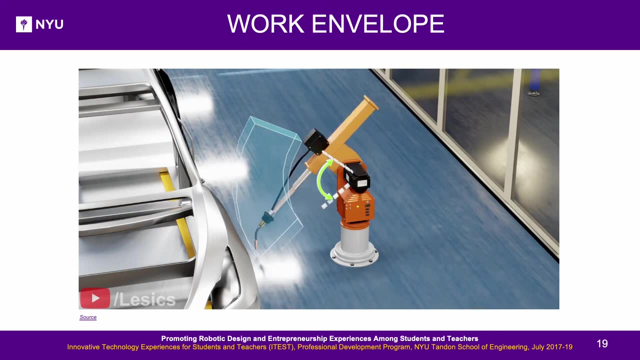 The cylindrical robot cannot perform this task. All you have to do to achieve it is replace one more linear joint with a rotary joint. Here. this rotary joint can go from approximately positive 30 degrees to the bottom of the ground. Now, using your visualization skill, can you predict this robot's work envelope? 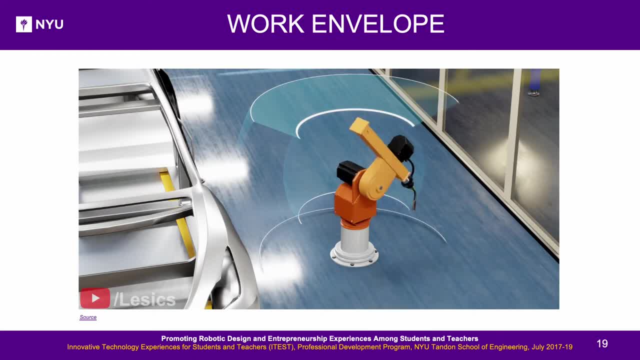 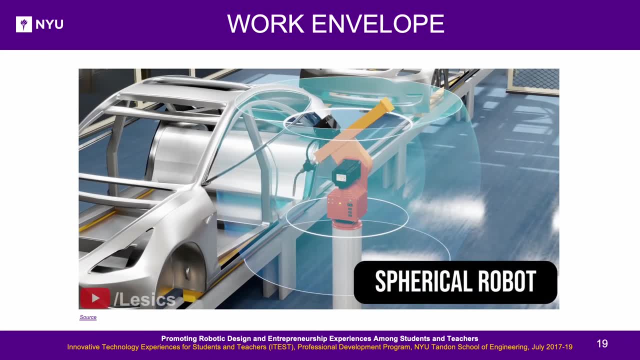 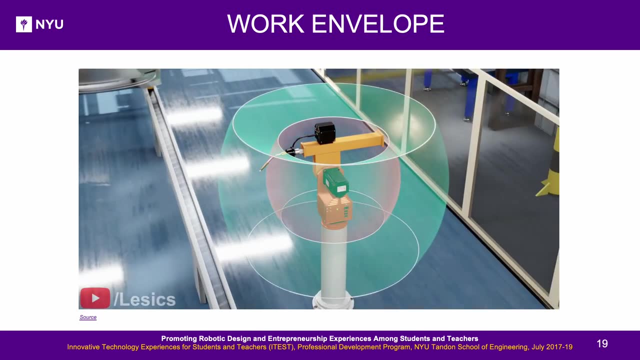 Just revolve this shape 360 degrees in the Z-axis. What you get is a partially spherical work envelope. These kinds of spherical robots can easily complete this welding task with an angle. What you see in the central area is the dead zone of a partial spherical configuration. 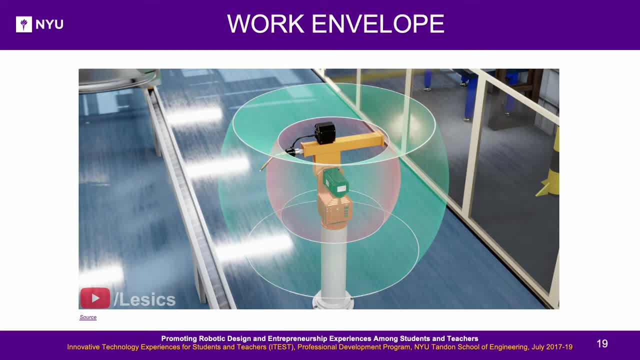 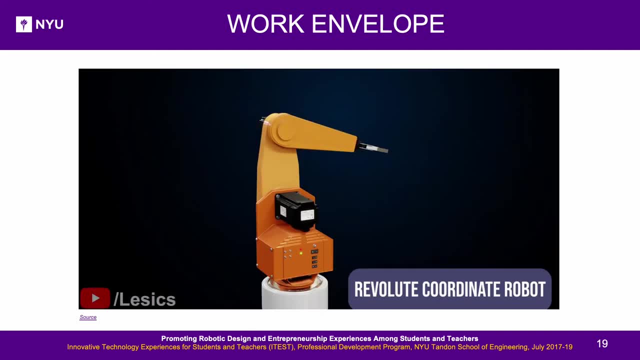 This space can be an efficiency weakness. If we replace the last linear joint from our bot with another rotary joint, this will make it a revolute coordinate robot, which should reduce the dead zone and give the bot more reach. This robot looks similar to a human arm right. 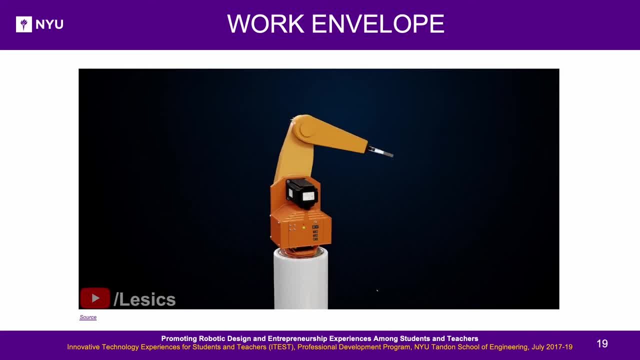 Now the new challenge. Let's deduce its work envelope. First, let's freeze the Z-axis rotation and figure out the 2D work envelope which arises due to the robot's remaining two rotary arms. When both the arms are fully stretched, the end effector can draw a circle of 280 degrees. 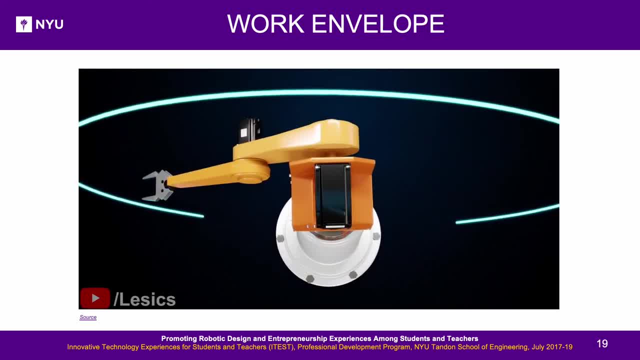 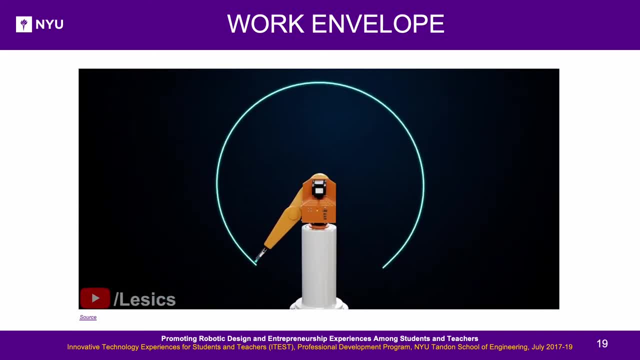 You can observe from the top view why this joint cannot go beyond this 280 degree angular limit. Anyway, this is the biggest circle this robot can draw. Now we need to figure out the smallest circle this robot can trace. This robot traces the smallest circle possible when the arms are folded like this. 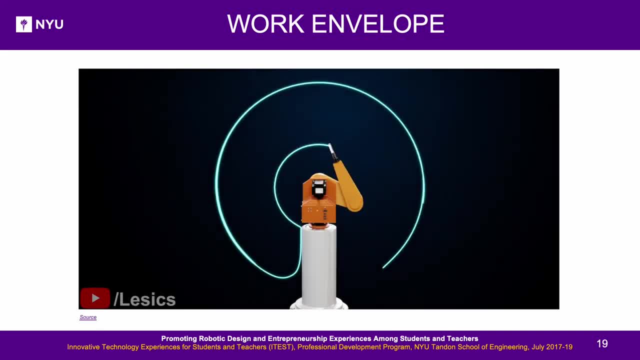 However, after a certain movement, the circle can't be traced further because the lower arm will touch the robot's body. The trick to extend the circle tracing is simple: Just fold the arms the opposite way. Now you can trace the circle further.